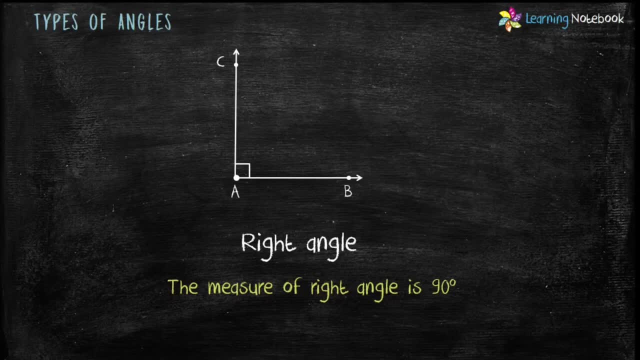 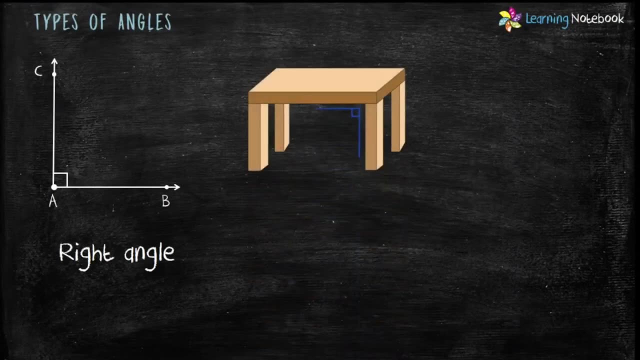 the figure. So here angle BAC equals to 90 degree. You may not notice, but right angles can easily be seen in our daily lives. Some of the real life examples of right angle are: first, a table Left of the table, right angle with table top. Left angle with арabic angle. 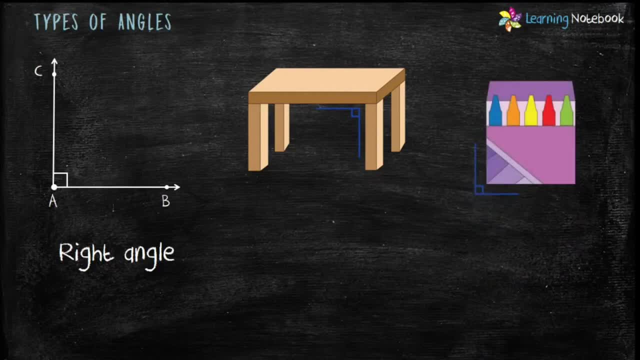 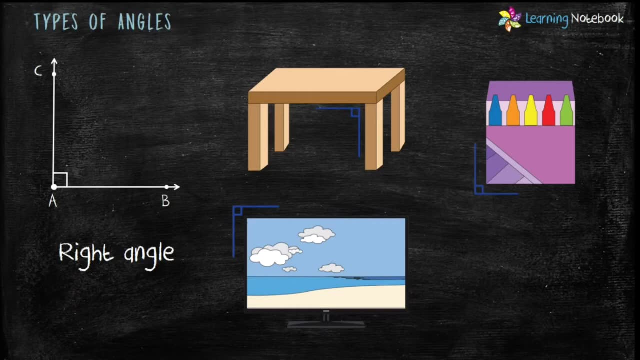 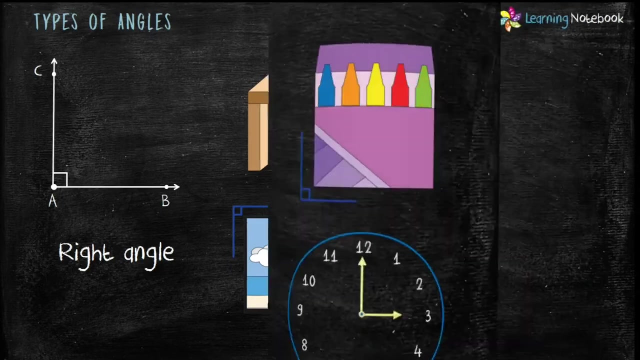 Second, your color box: They make right angle. Third is a television set, Edges of television set. they make right angles. And fourth, the clock. The hands of the clock make right angle at 3'o clock. Second type of angle is acute angle. 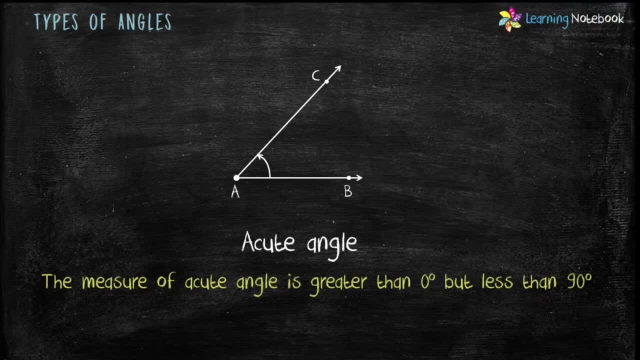 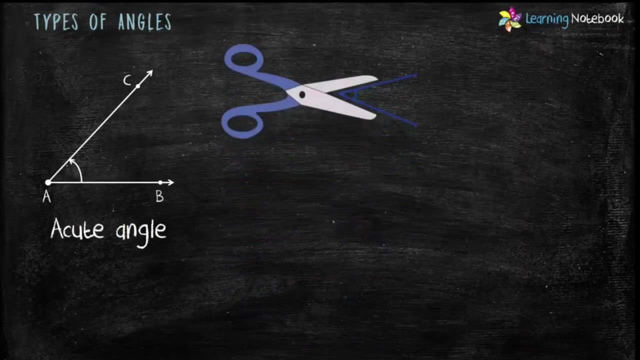 And the measure of acute angle is greater than 0 degree, but less than 90 degree, as shown in the figure. So here, angle BAC is an acute angle. Students, let's see some real life examples of acute angles. First is pair of scissors. 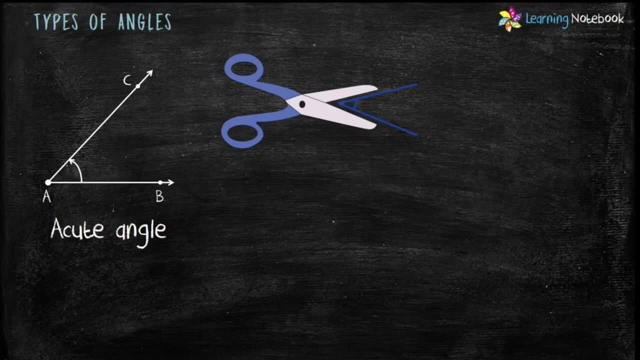 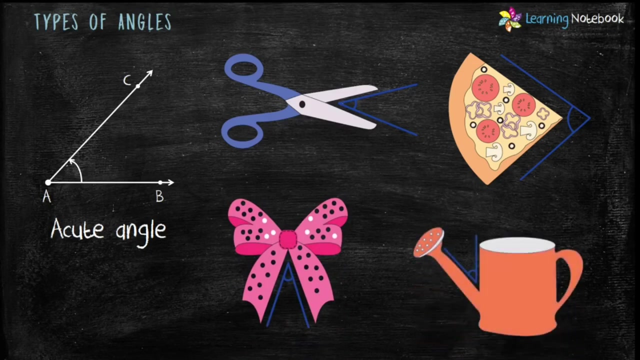 Blades of open scissor make an acute angle. Second, a pizza slice. Edges of pizza slice make an acute angle. Third, a bow. It is making an acute angle. And fourth is the gardener jug. It is also making an acute angle, as shown here. 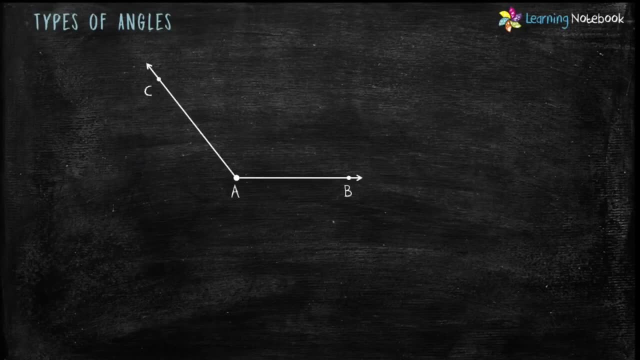 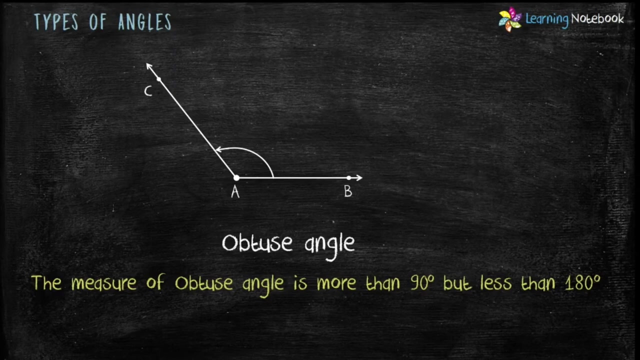 Now, third type of angle is obtuse angle And the measure of obtuse angle is more than 90 degree, but less than 180 degree, as shown in the figure. So here angle BAC is an acute angle. So, students, here angle BAC is an obtuse angle. 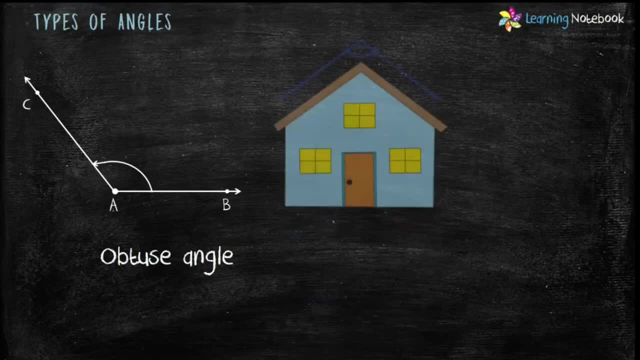 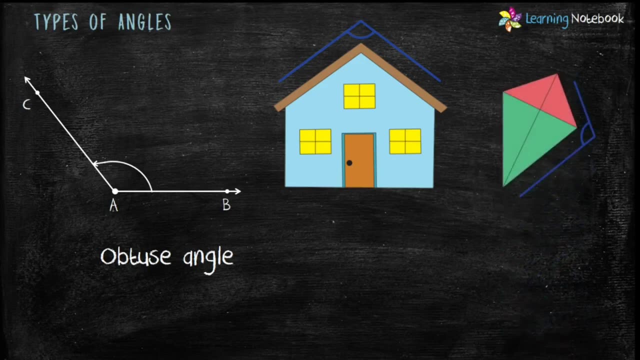 Now let's see some real life examples of obtuse angle. First is house roof: It makes an obtuse angle. Second is a kite. Edges of kite make an obtuse angle. Third is Japanese fan. When we open such a fan, it makes an obtuse angle.